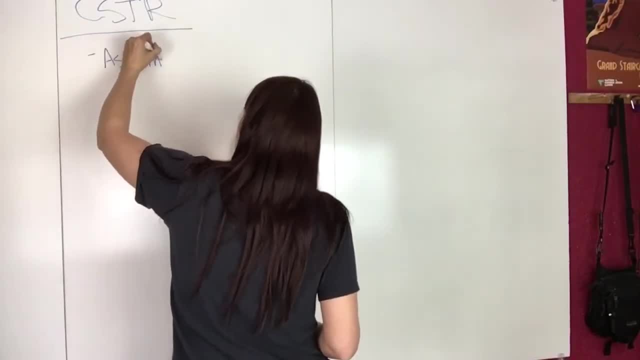 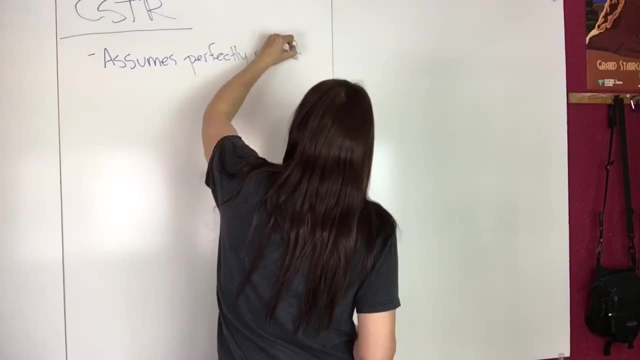 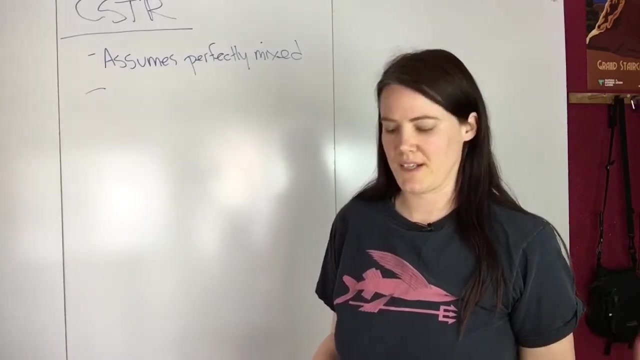 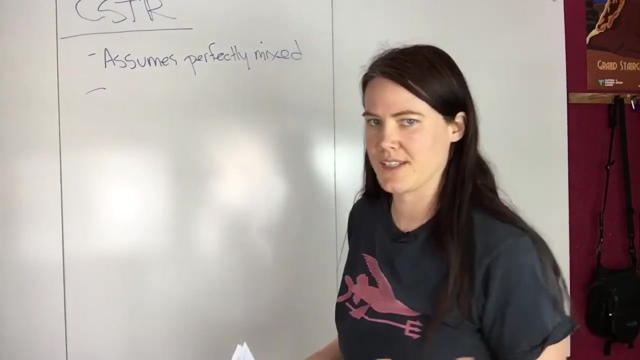 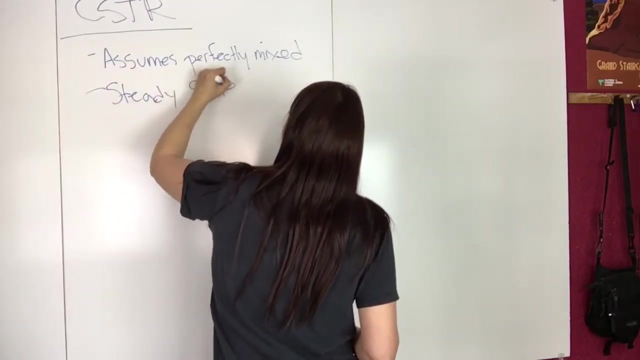 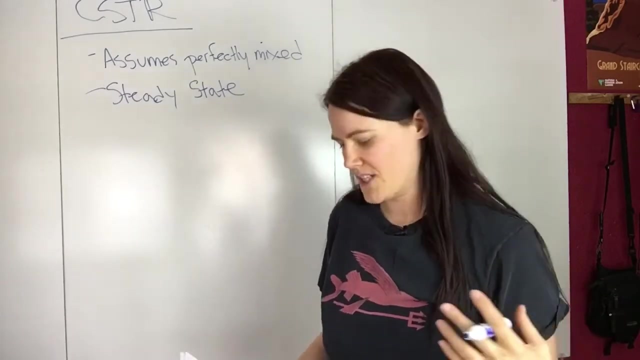 perfectly mixed, And it also assumes that it's operated at a steady state, So there's no dependence on concentration or no time dependence on concentration or temperature and stuff like that. So steady State. So then, if I write down the general mole balance equation that I derived in a previous 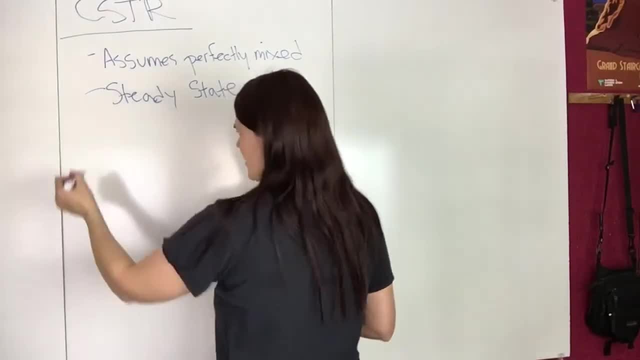 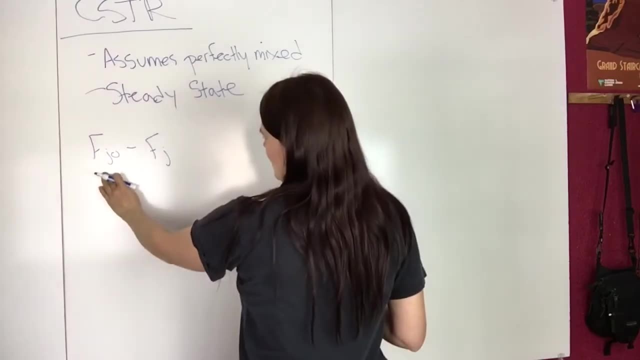 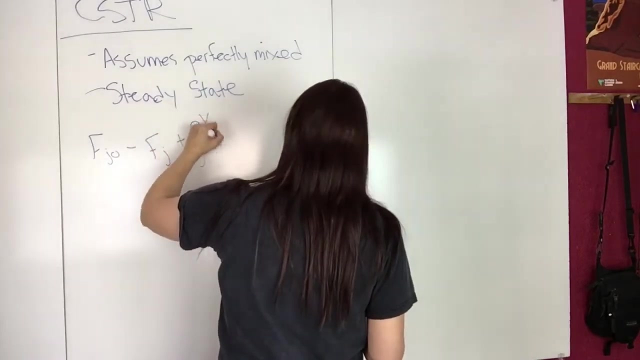 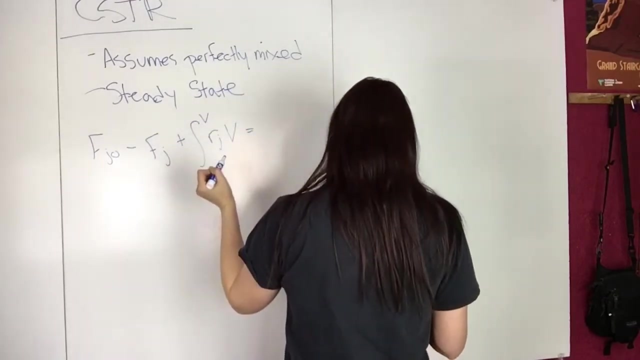 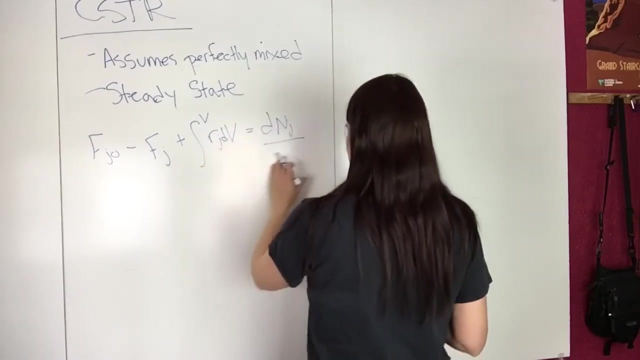 video I'll get this. So this is the general mole balance. So FJ naught minus FJ. So whatever's flowing in minus whatever's flowing out plus what you're generating inside the reactor. I thought something looked weird. D And then this is what is accumulating inside with time. So 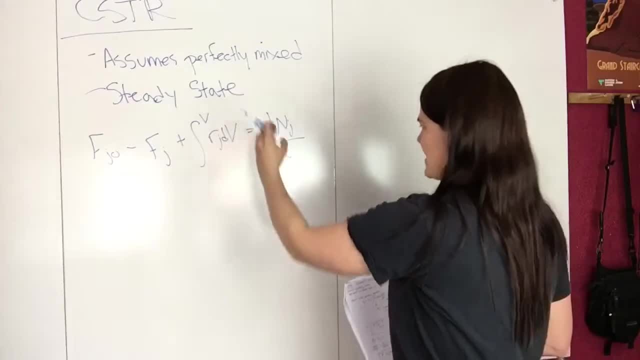 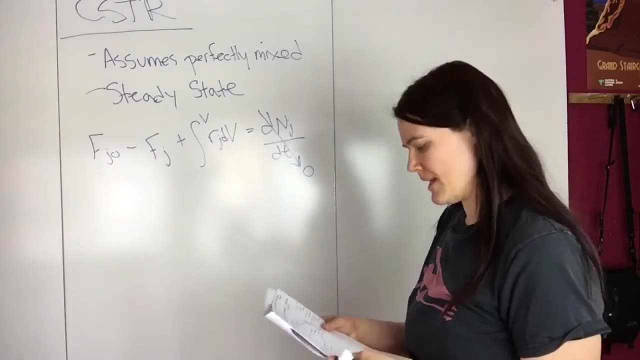 looking at this, first of all, we know that, since it's steady state, this term is zero, Because there's no dependence, There's no change, There's no dependence on time. And we also know that there, since it's perfectly, 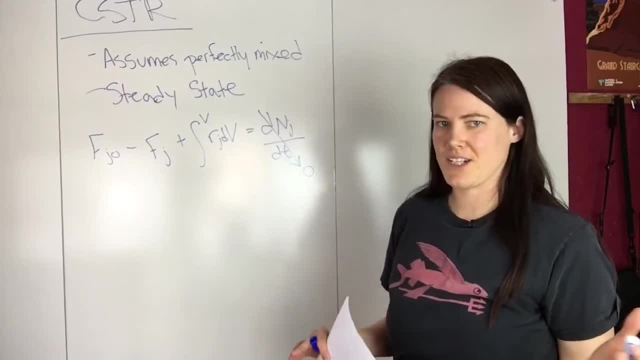 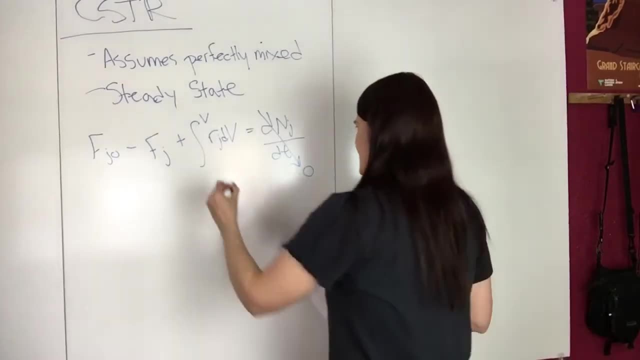 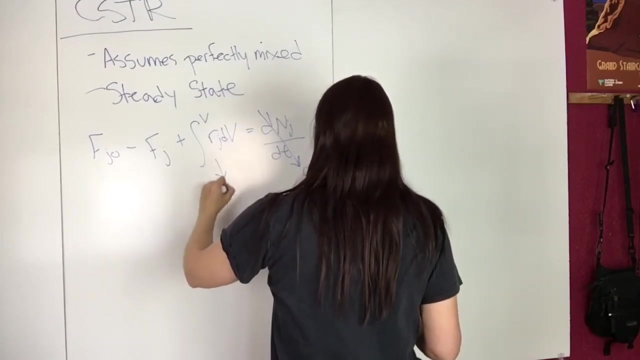 mixed, there aren't any spatial variations with the rate. So for instance, it's not. the rate isn't dependent on position, And so then you can pull this out of the integral also. So then you would end up with RJV. 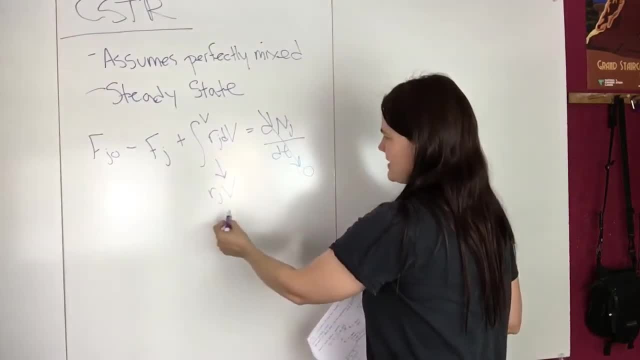 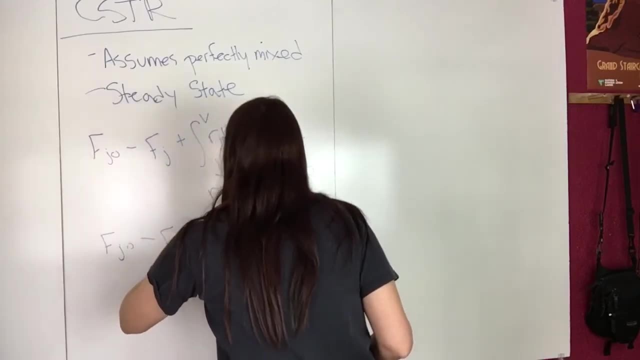 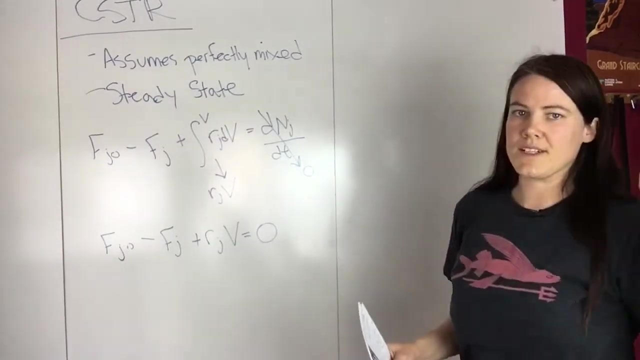 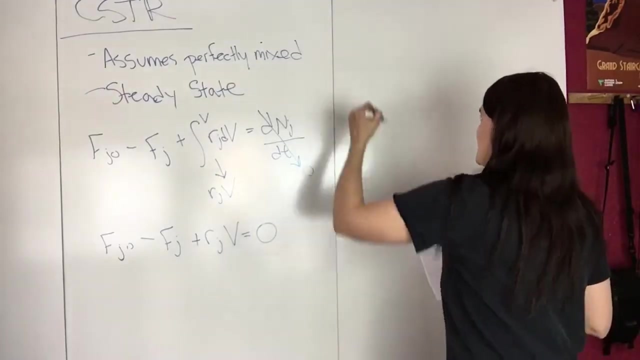 So then you can rewrite this equation. So FJ naught minus FJ plus RJV equals zero. And then what we want for this, what we want for this equation, is the volume. So we can go ahead and solve for volume, So you end up with: